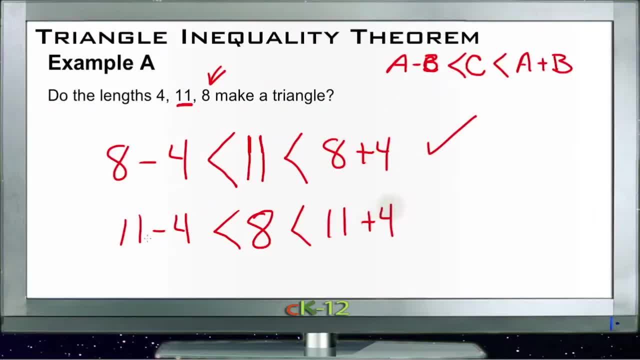 of 11 plus 4.. 11 minus 4,, of course, is 7,, that's less than 8, and 8 is less than 15.. So yeah, this definitely makes a triangle. no problem, Let's take a look at example B. Example B says: find the length of the third side of. 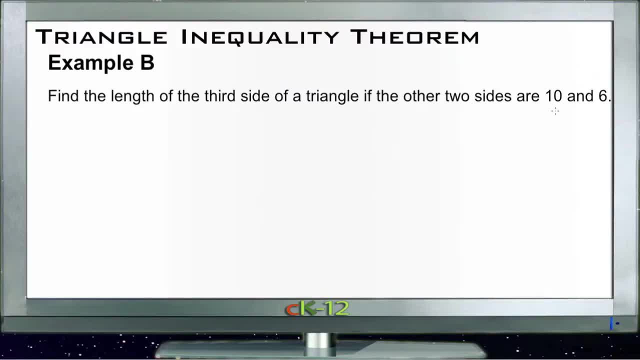 a triangle if the other two sides are 10 and 6.. So we're missing side C and we know that it has to be greater than the difference between 10 and 6, but less than the total of 10 and 6, plus 6.. So C must be greater than 4, but less than 16.. So anywhere between you know. 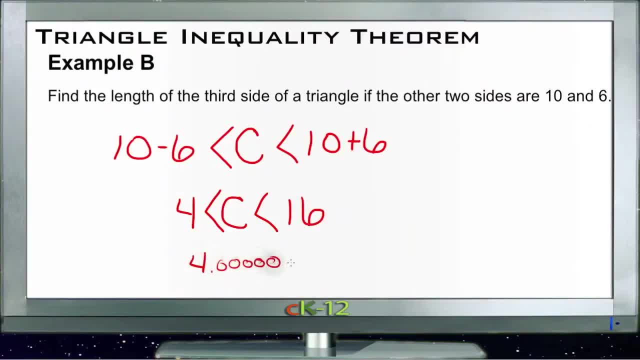 4.000000, forever, as long as you want 1,, and all the way up to 15.9999999999, as long as you want. It can't quite be 16, and it can't quite be 4.. 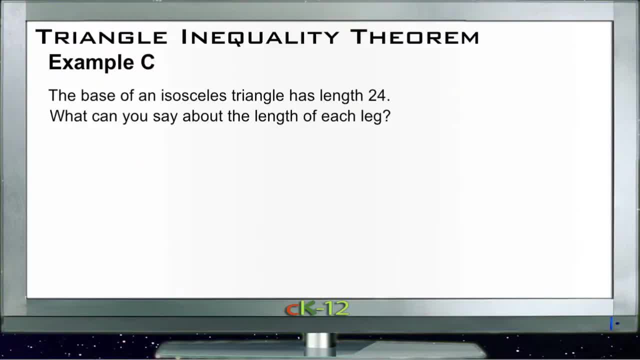 But anywhere in between is fine. And then, finally, let's take a look at example C. Example C tells us that the base of an isosceles triangle has a length of 24.. What can we say about the length of each leg? So? 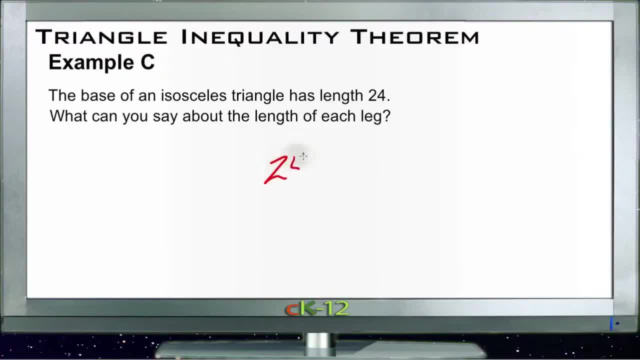